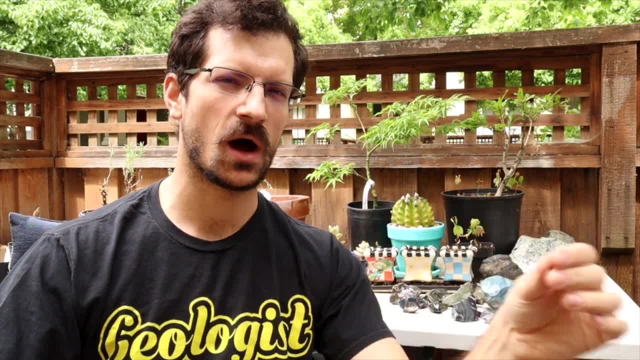 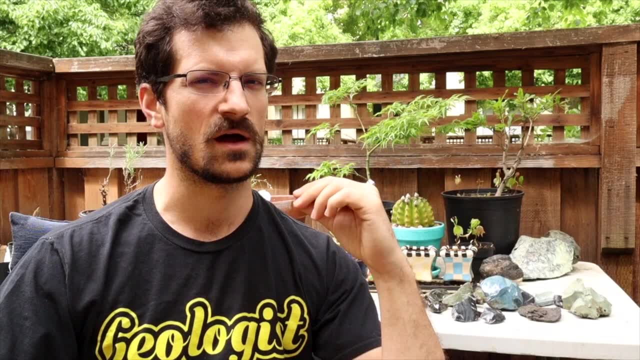 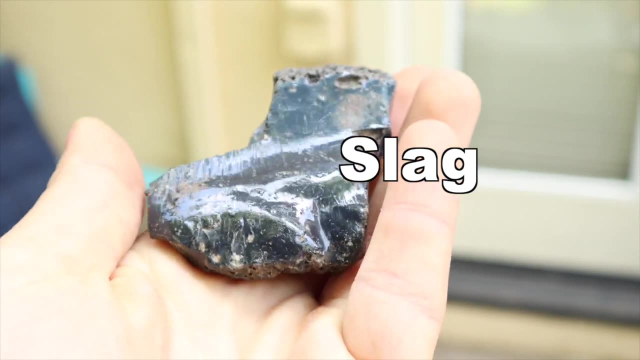 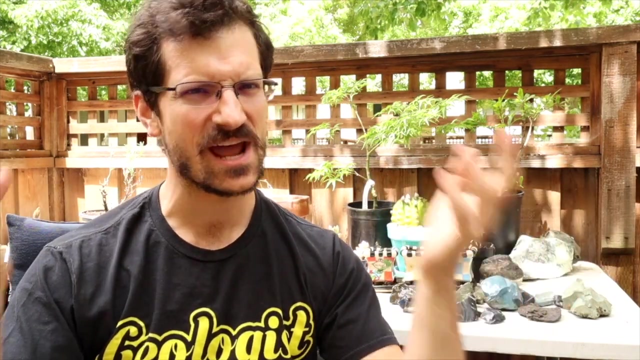 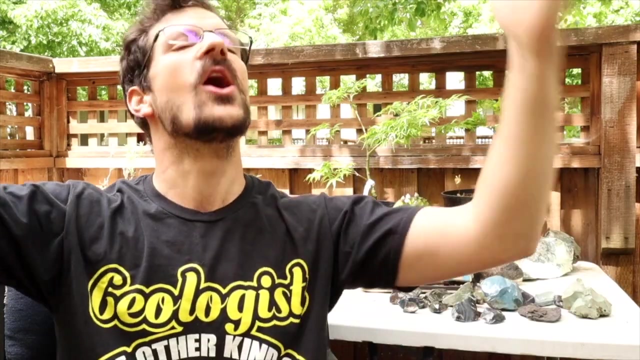 One of the most common mistaken rocks that I have seen on the internet and especially on the subreddit. what is this rock is the difference between slag, glass and obsidian. So today, rock stars, I want to talk a bit about what is slag, What is obsidian, How are they similar and how are they different and how you can tell the difference. on this episode of Brock talk: 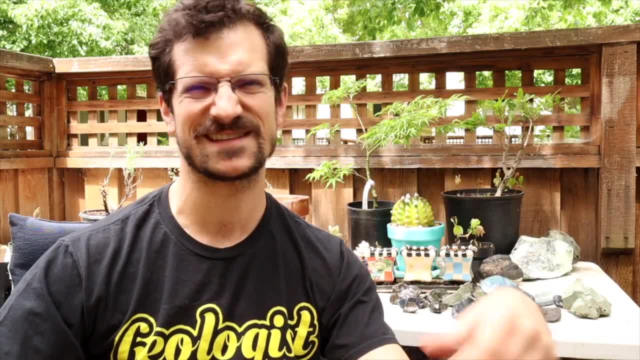 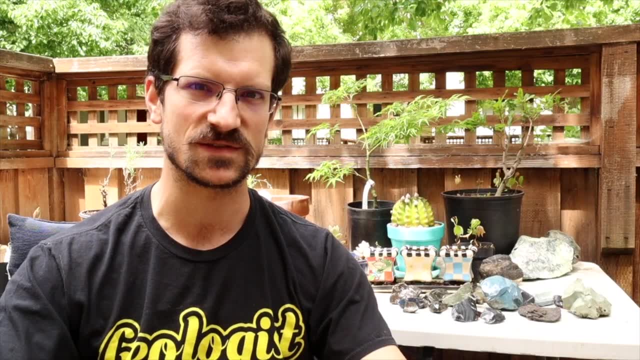 Slag glass is an industrial waste product. It is a byproduct typically of metal foundries when you are making steel or other kinds of metals. Basically, all it amounts to is a silica with a metal base, A little bit of metal in it. 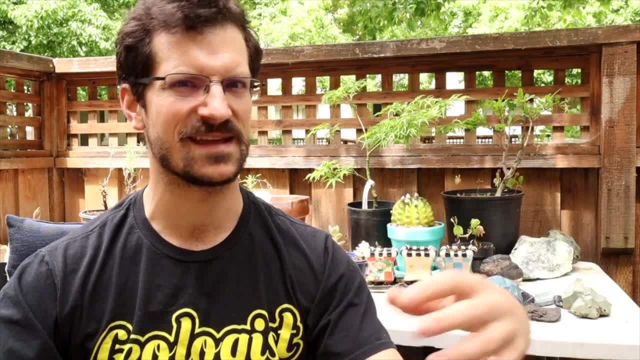 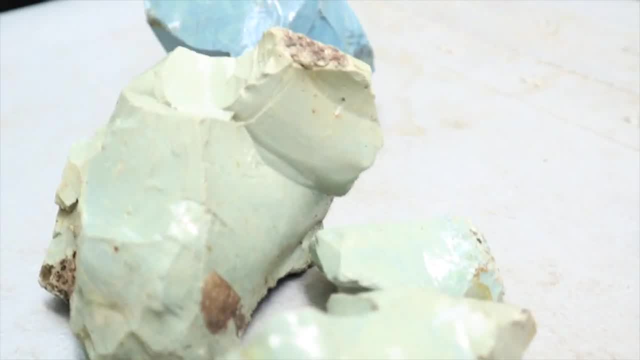 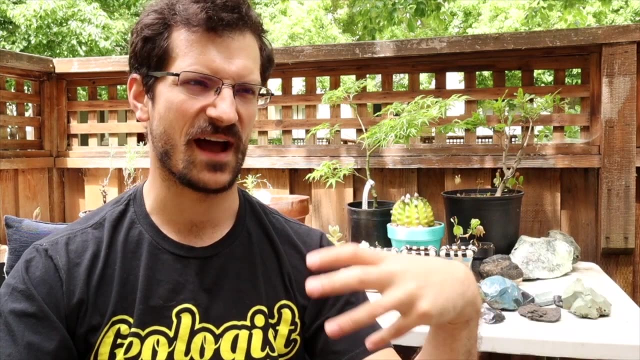 And that amount of metals and other impurities in that silica will change the color of that glass into all kinds of different colors. You can have slag glass of beautiful, gorgeous, vibrant colors that also will shatter like glass. So it will have a typical conchoidal fracture and it will also form very sharp edges. 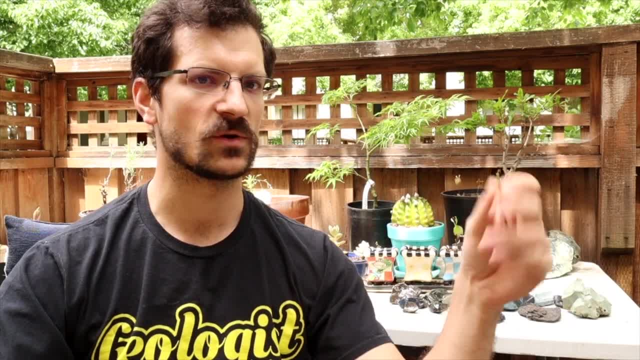 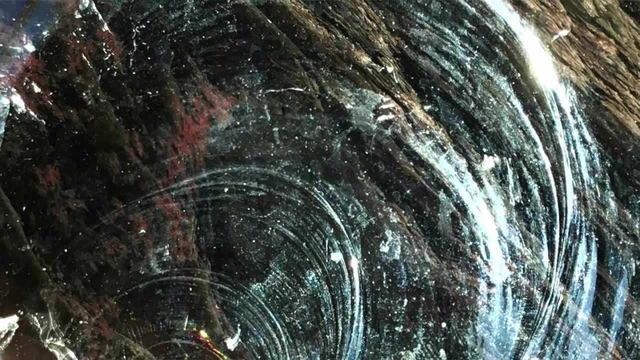 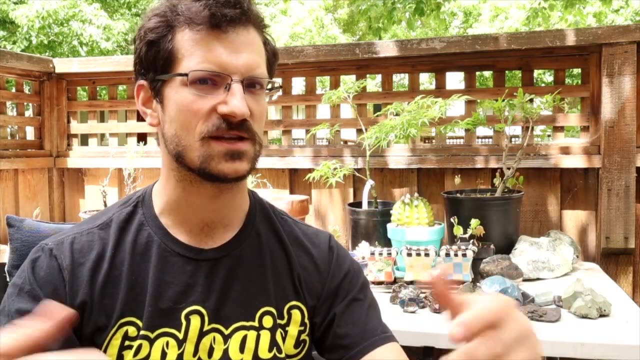 Now, those are all things that people can also associate to obsidian. to a certain extent, Obsidian can sometimes have very vibrant colors, shatters and has that conchoidal fracture. But unlike slag, it is not an industrial made rock, It is a. 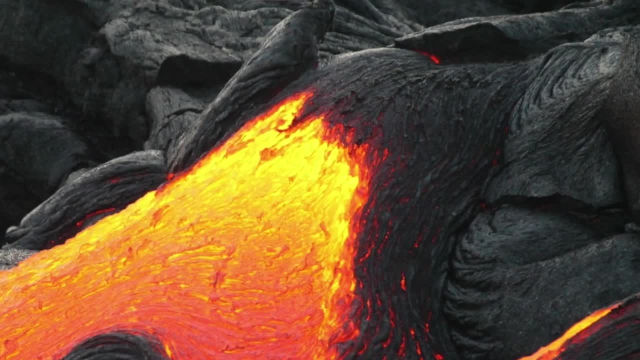 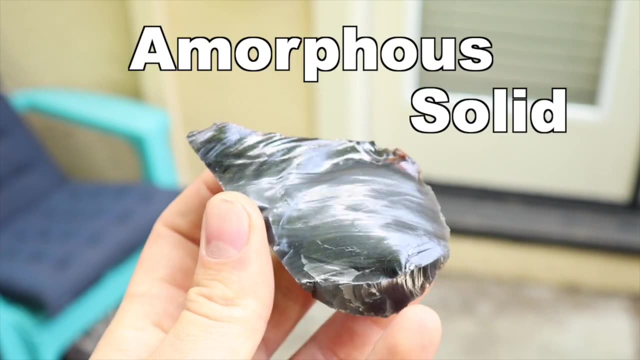 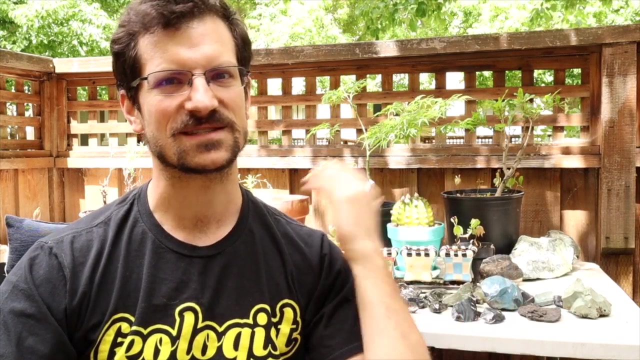 naturally forming silica glass that comes from volcanic processes that cool on the surface very quickly, creating an amorphous solid like glass. Totally awesome. I featured it in a video years ago when we smashed the crud out of a piece of obsidian glass- Totally. 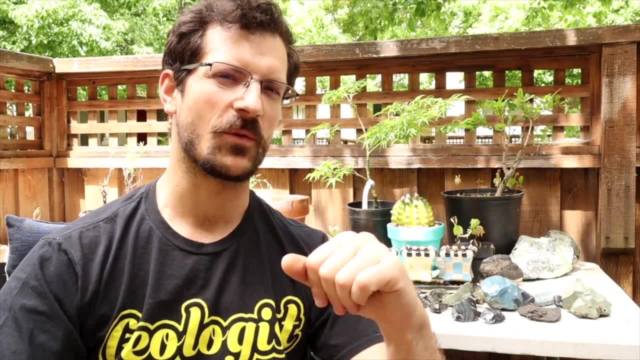 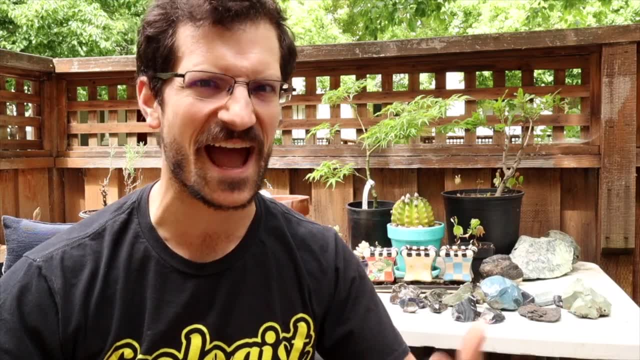 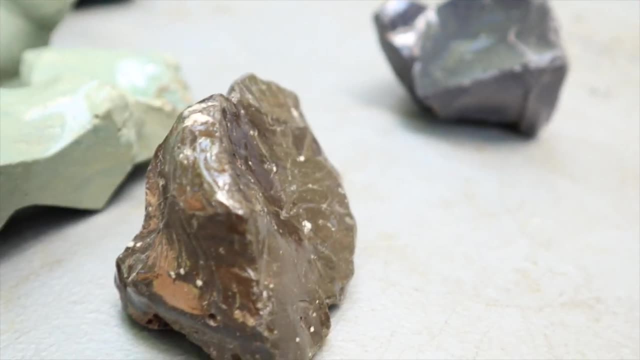 awesome video And if you want to check that out, I've linked that up here in the upper right hand corner. So for a lot of beginning rock hounders, when you find a piece of slag you feel like you hit pay dirt man, Like I found a bunch of these colorful rocks. They 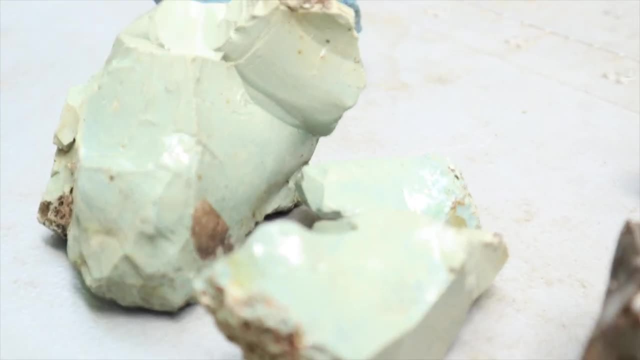 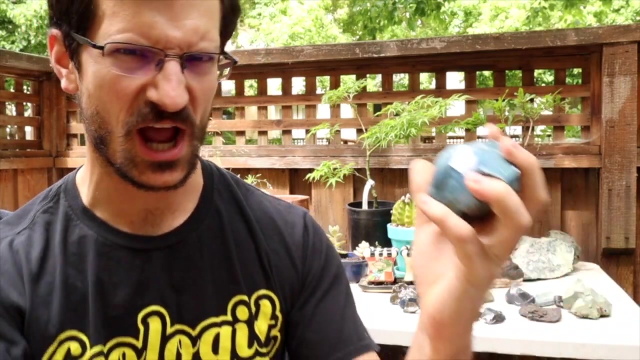 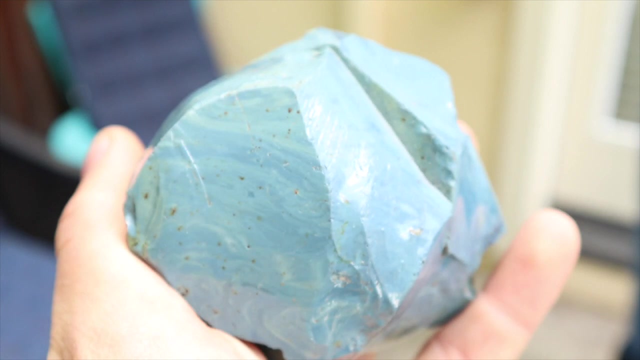 were so bright and vibrant. And then I found the mother load. I found this blue gemstone. It just looked absolutely beautiful. It had all these swirling patterns, It had what looked like conchoidal fracture, conchoidal fracturing- And it just 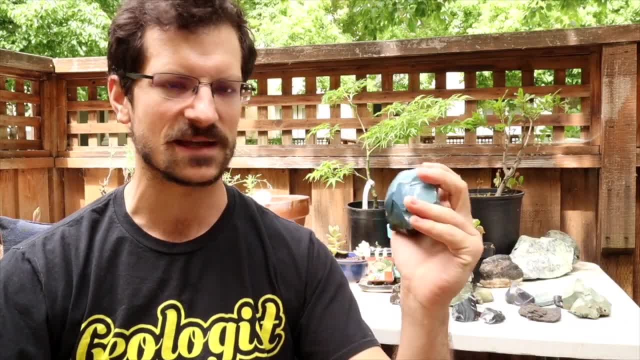 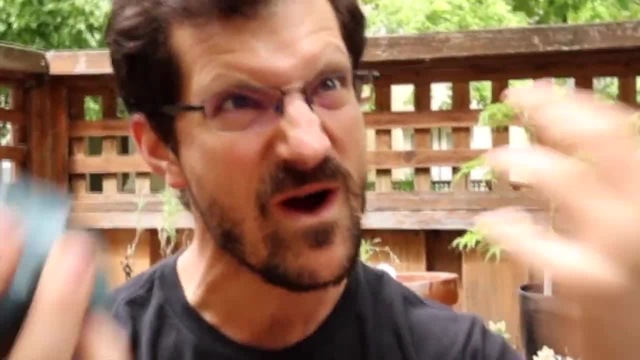 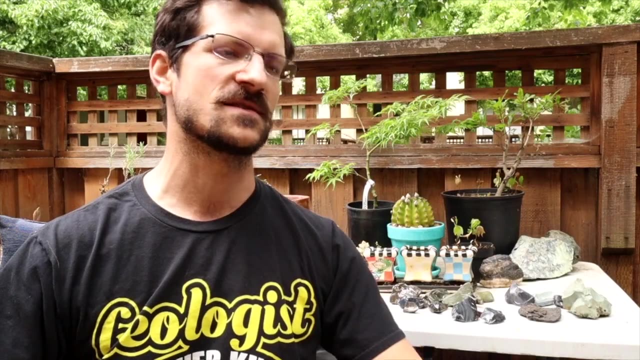 had that sheen that looked almost exactly like glass. I thought I hit the jackpot. I thought here I am sitting on this awesome rock. I was like, wow, Oh my gosh, I just found the coolest piece of obsidian Ever Million years. Wouldn't think I'd find something so cool, Totally awesome. And then I 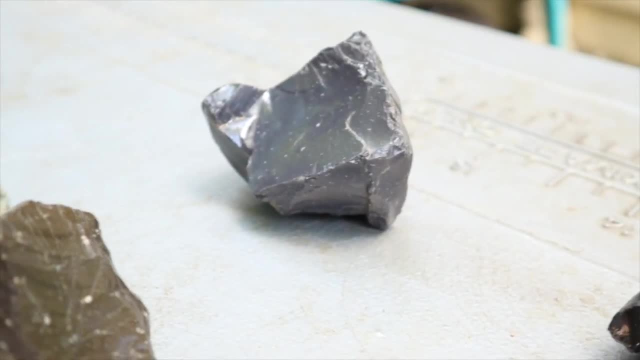 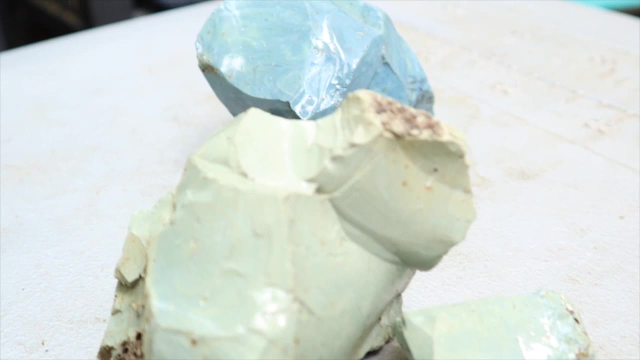 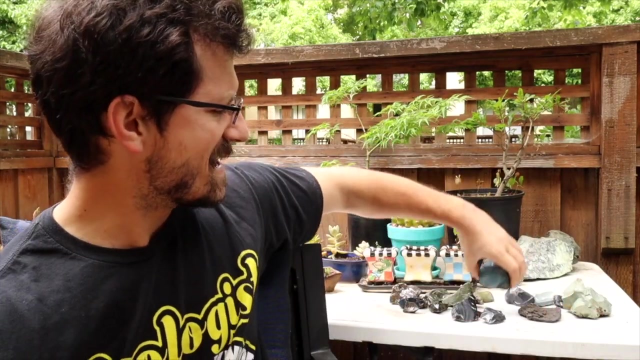 looked into it a little bit more, Turns out this and the other pieces that I found and thought were obsidian are all slag glass. But what makes the difference? What's the big hoop between this and a piece of obsidian? The devil is absolutely in the details. on this one, They're rock stars. You. 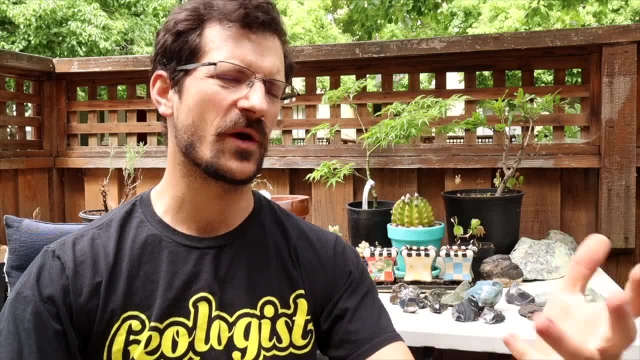 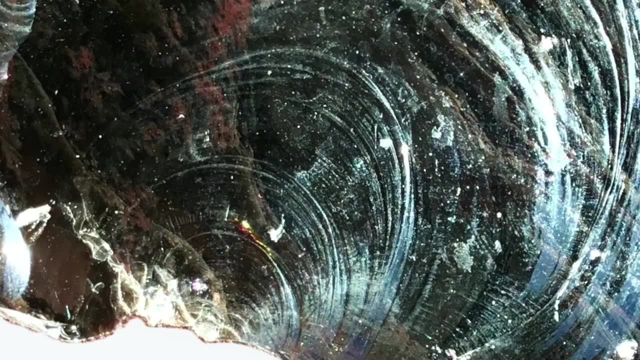 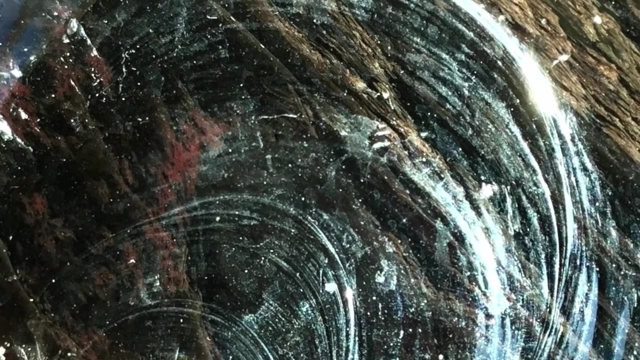 know they're a couple different factors. So you know we can't use conchoidal fracture to rule out either of these two rocks. And very simply, conchoidal fracture is just that wavy pattern, that undulating pattern that appears on obsidian and other kinds of glass when it's struck. 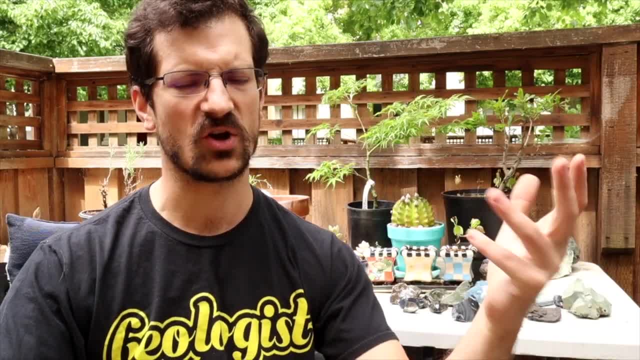 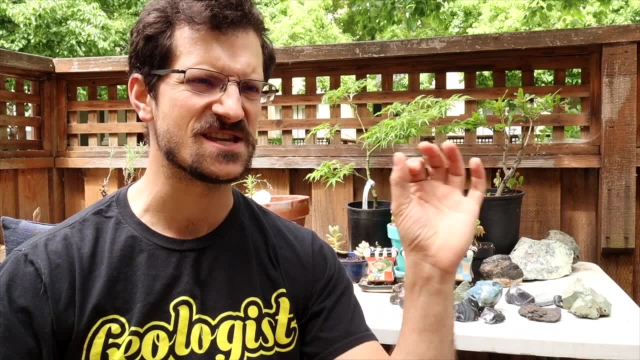 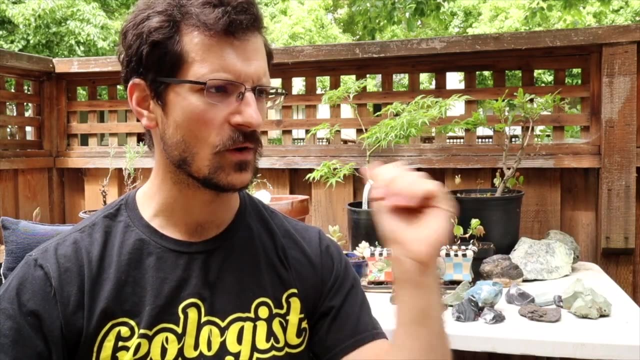 when you hit it, when you crack it open, Both slag and obsidian are going to have conchoidal fracture, so it's not going to be very useful. There are, though, a few very key differences, these two rocks, that we can use to better nail things down. For the most part, though the most 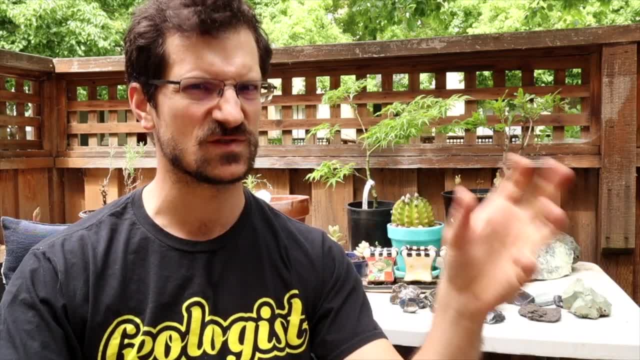 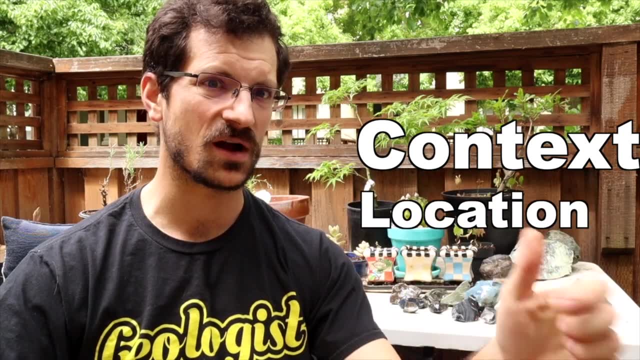 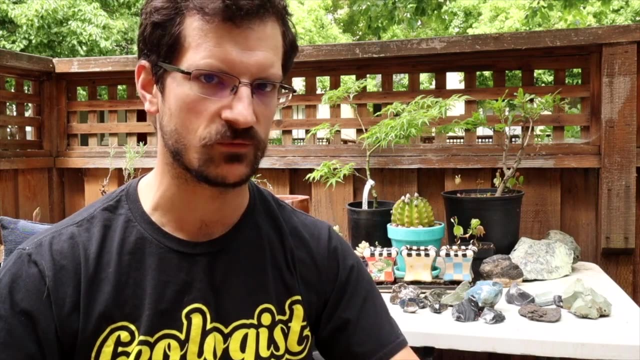 important thing to consider when you're trying to identify between these two rocks is the context in which you found that rock, Both the location of the rock and also the placement of the rock that you found it. Did you find your mystery rock on the side of a hill? Was it buried in the dirt or 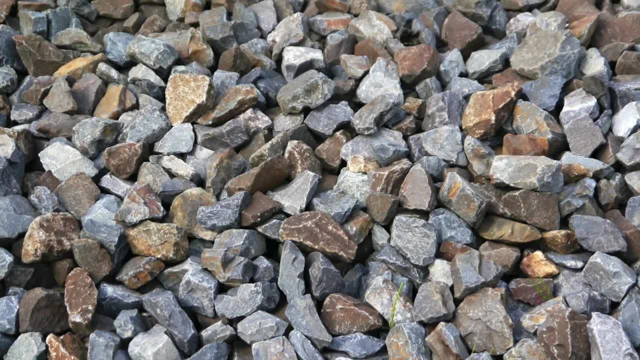 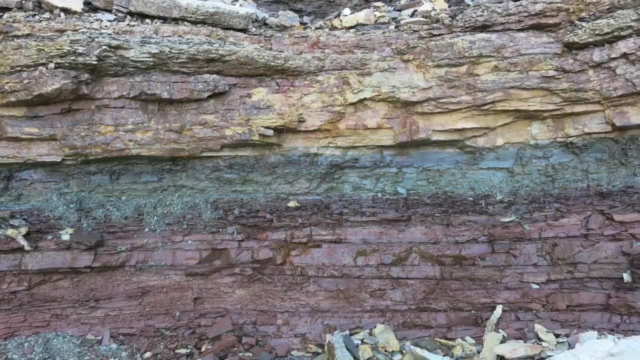 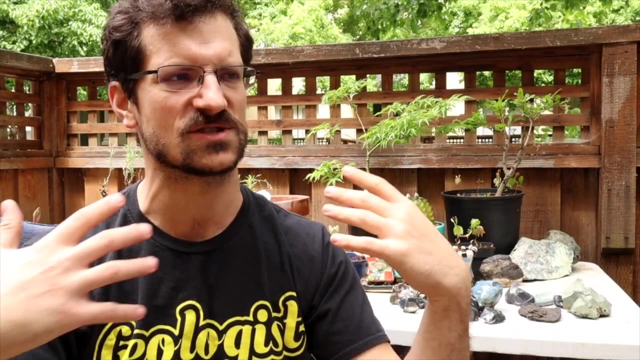 was it just sitting out on top? Was it in a pile, a big piling of glass, other glass shards, or was it in a thin bedded deposit? These are going to be really important things to take note of, both as a scientist and a geologist, or even just a rock hounder, that you're going to want to keep in mind. 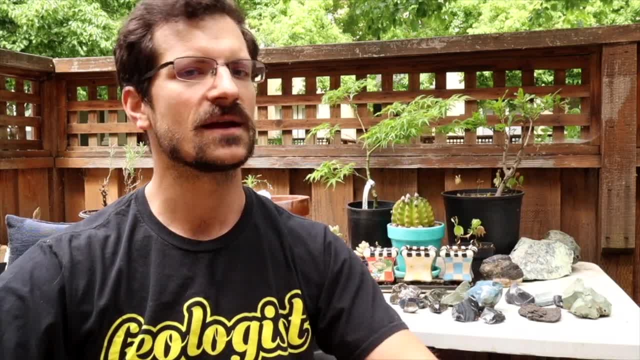 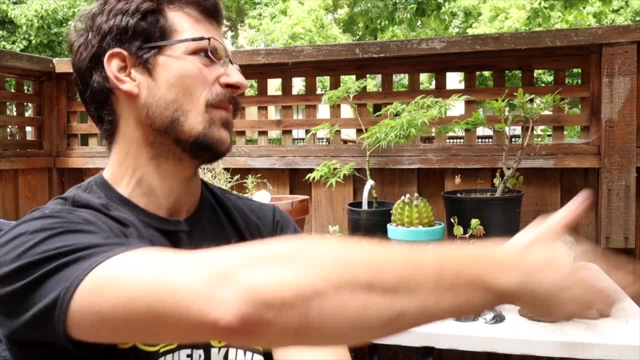 because the context of how you found it and the location can tell you a lot as well. In case you didn't notice, rocks don't move very far, they don't have legs, They can't just get up and walk somewhere else. So, wherever you put them, wherever you set them down, 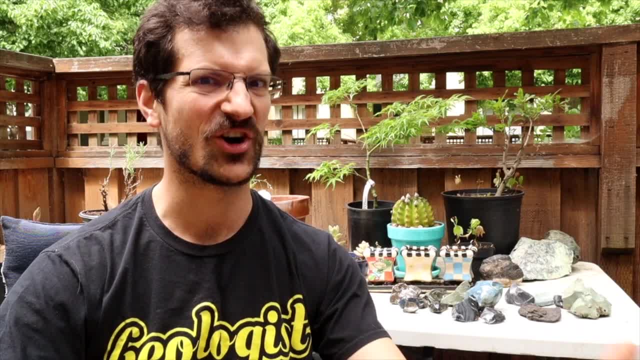 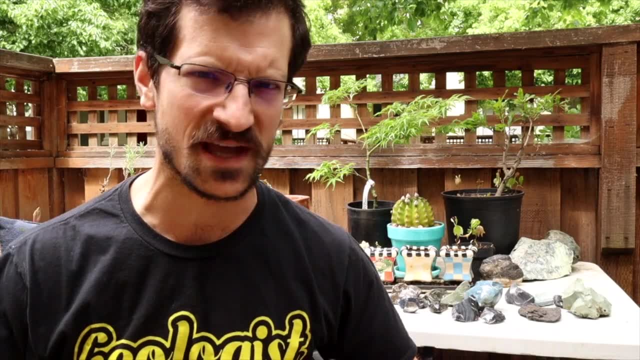 They're gonna stay there for a very, very, very long time. So if you're in an area that has absolutely no volcanic deposits at all, You don't have any volcanics at all in your local area. It's that rock that you found that's really shiny and looks like glass. 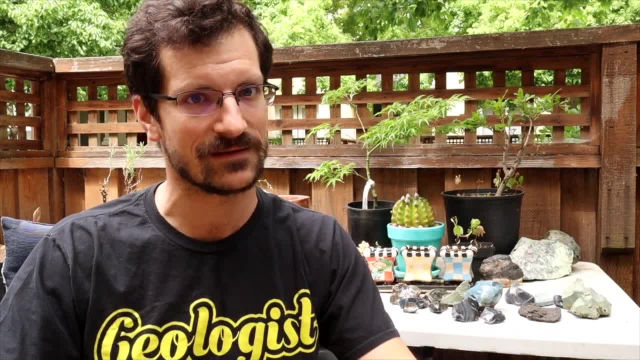 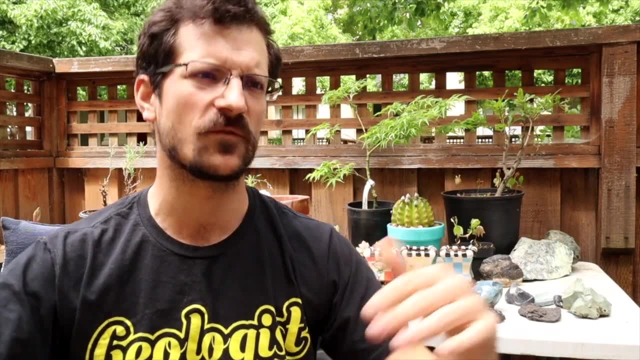 Probably isn't going to be obsidian. just because it's unlikely now, that doesn't rule out Some very rare cases where it can be. but that's just kind of the first checks You want to be doing before you get to the more final details of really identifying that rock. 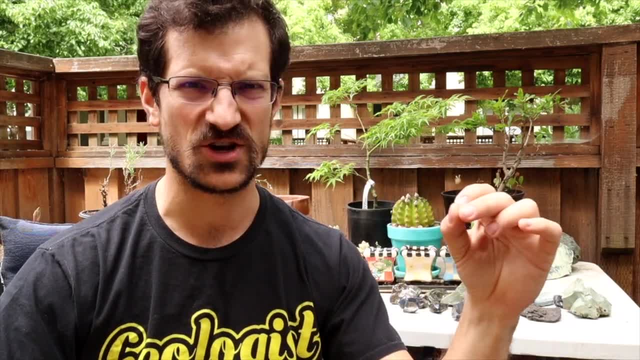 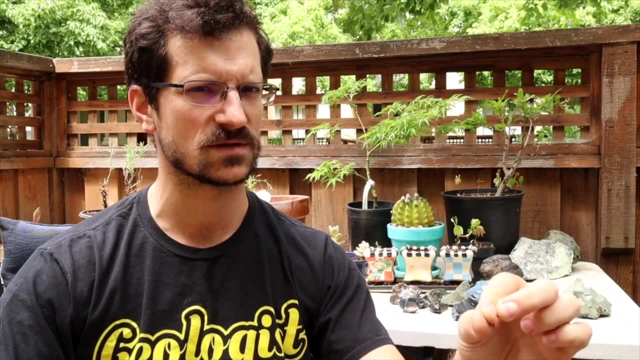 Let's say that you've narrowed it down. You know that you've got volcanics in your area. You know that that Obsidian is possible. It's a possibility. How do you rule out whether it's slag or not? And for that, you know, really want to take a look at some of the pieces that you picked up. 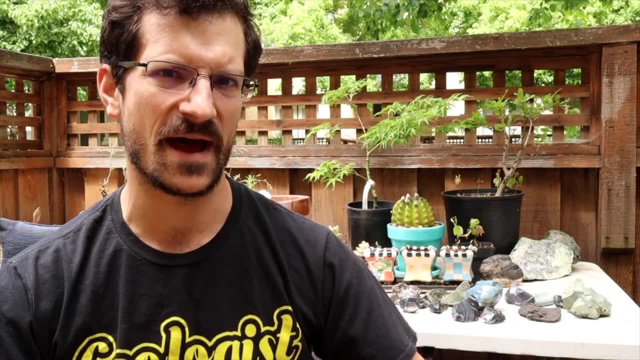 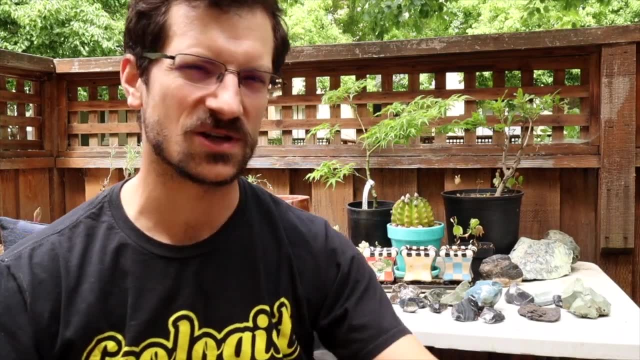 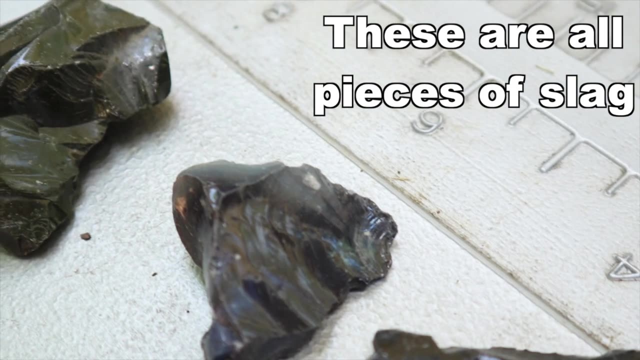 Slag is going to form in a number of different Patterns in a given deposit and then given slag heap. basically, as a result, You're gonna see all different kinds of colors of slag, but also all different kinds of patterns as well. Slag glass can very typically have lots of swirling colors in it- very attractive swirls of color. 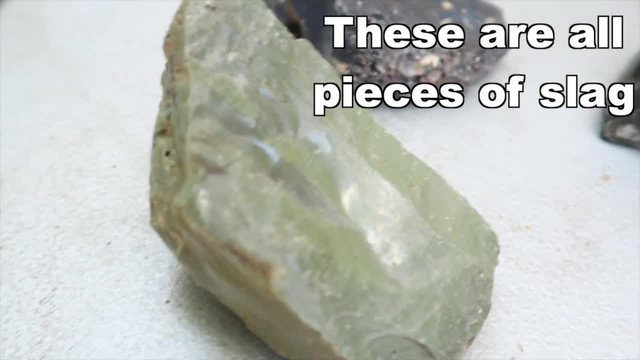 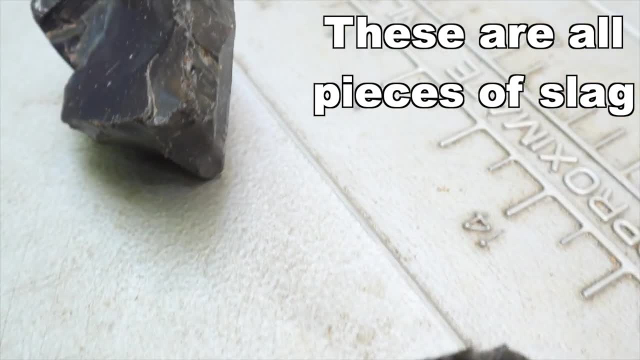 Or it can also have just very vibrant, extremely vibrant colors relative to obsidian, Which is most often going to be black or brown in color, the two most common Colors there. so the very first thing: if you have very brightly colored piece of glass, it might not be. 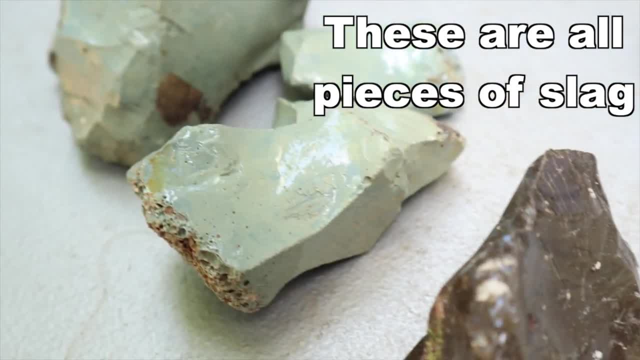 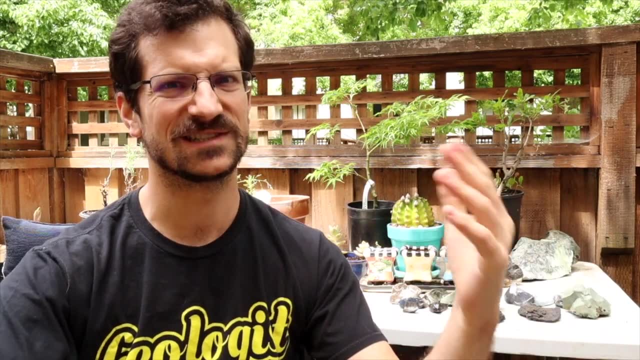 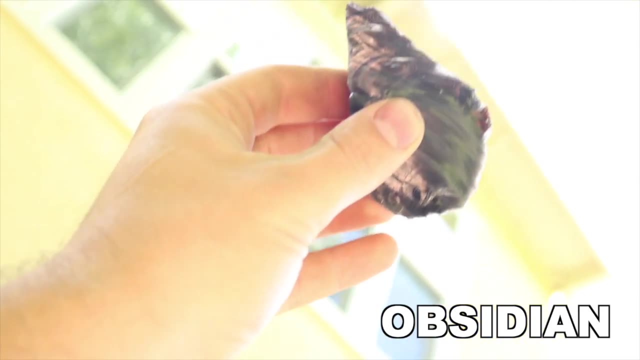 Obsidian. the chances are low, but it could be a very rare type. the next thing you're going to want to do is hold up your piece of glass to a light source, Because obsidian will let a little bit of the light through, especially on the thinner edges. the thinner edges of the obsidian. 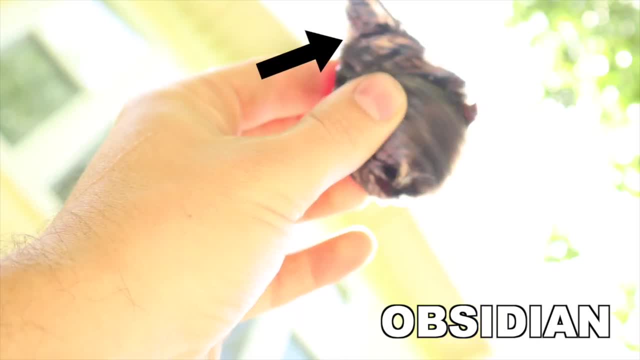 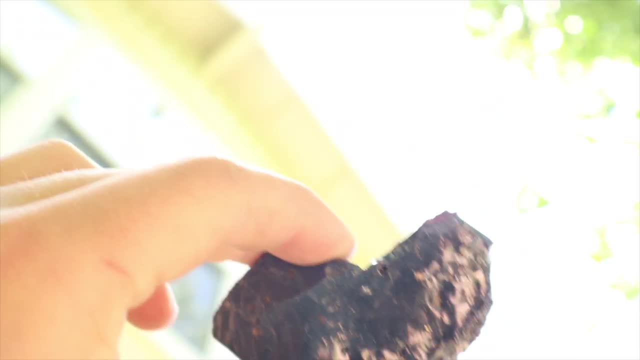 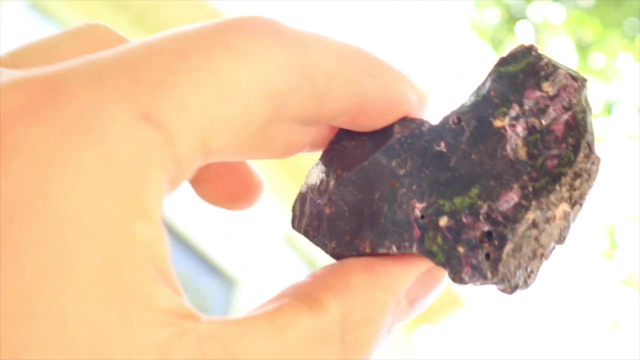 Will allow a little bit of light to pass through That rock, to pass through the crystals there, whereas slag is completely opaque, It won't let any light through at all. so that's going to be a very important distinction. That slag glass is not going to have those opaque edges like obsidian does. the next thing you're going to want to look for when? 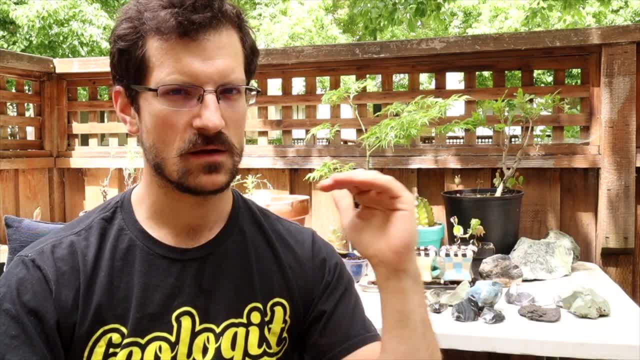 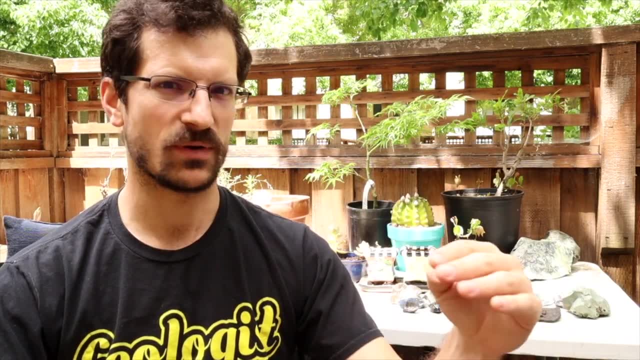 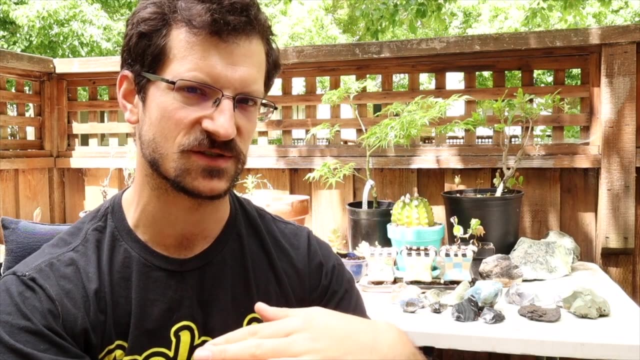 identifying your Glass is where that slag may have contacted the ground, because when they are pouring out slag glass at As a part of the industrial process, Oftentimes they're just pouring it on the ground or they're pouring it out on asphalt and that contact surface will have dirt. 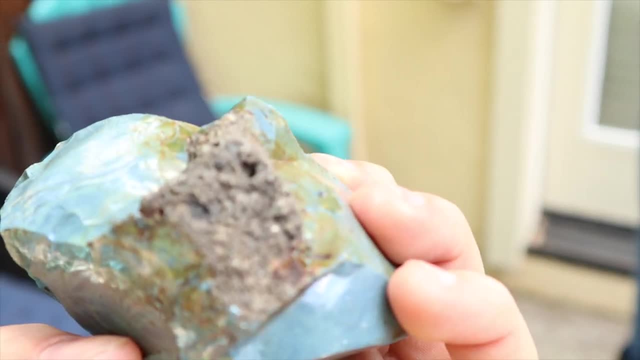 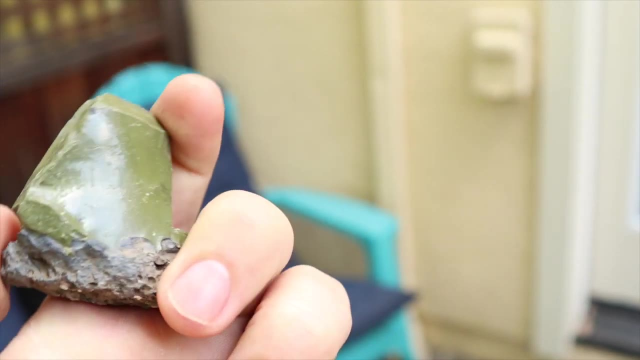 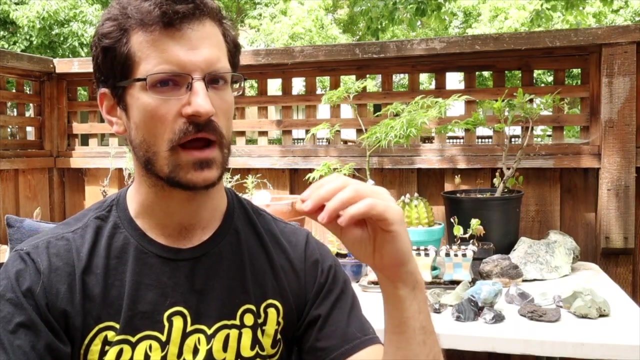 they'll have asphalt chunks or little pieces of Debris and sand. they get stuck Underneath that glass and is present in that final slag glass once It's all broken up and in a pile. so if you see that, it's a surefire sign that you're not looking at obsidian another really. 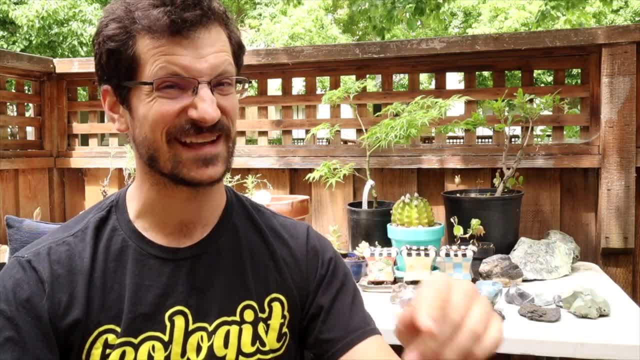 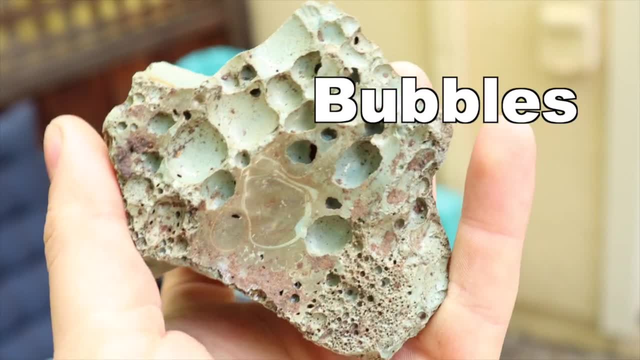 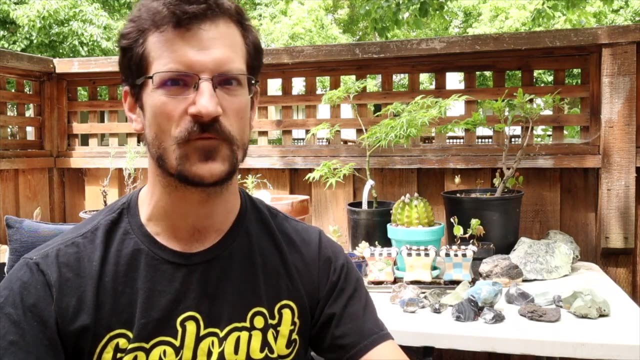 Critical key piece of evidence that you're looking at slag glass and not obsidian is the presence of bubbles. the entire definition of obsidian as a siliceous, Surfacial igneous rock. we just means that it's an igneous rock that forms on the surface and it has a lot of silica in it. a 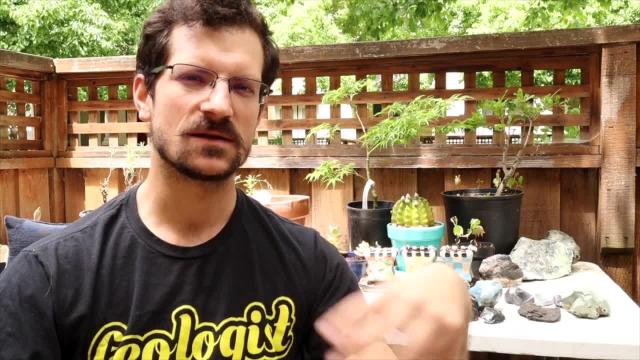 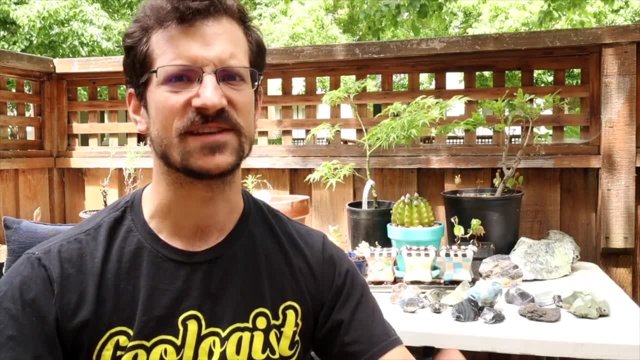 Lot of quartz is that that obsidian doesn't have a lot of gas bubbles. It doesn't have a lot of air bubbles in it when it forms. if you have too much frothy, Dissolved gases in a lava, when it gets to the surface It's not going to form an obsidian anymore. 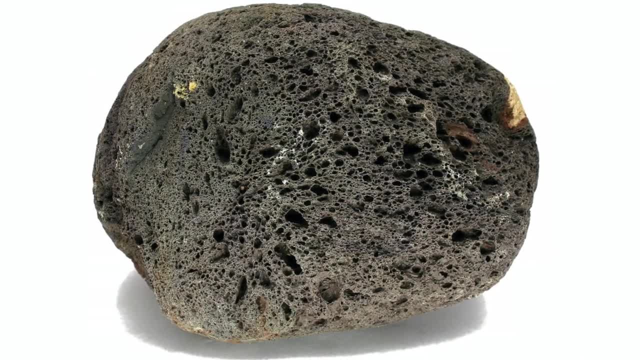 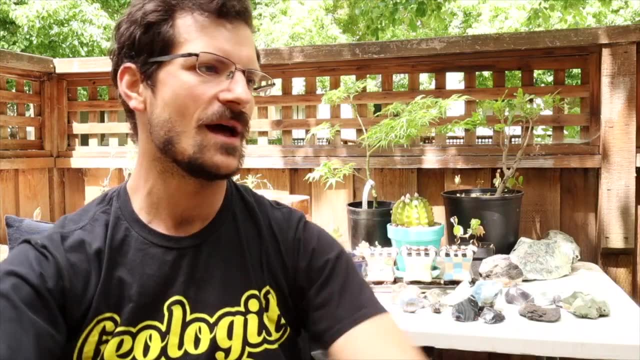 It's going to form a scoria, and scoria's are these big Bubbly masses of liquid rock that froth up like when you shake up a soda. can you pop that open? They're really cool- one of my favorite kinds of volcanic rocks- but they're not. 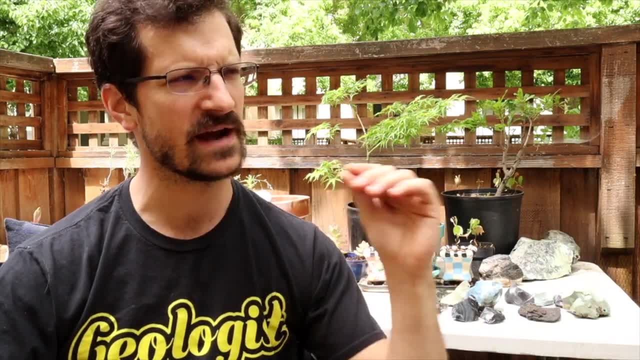 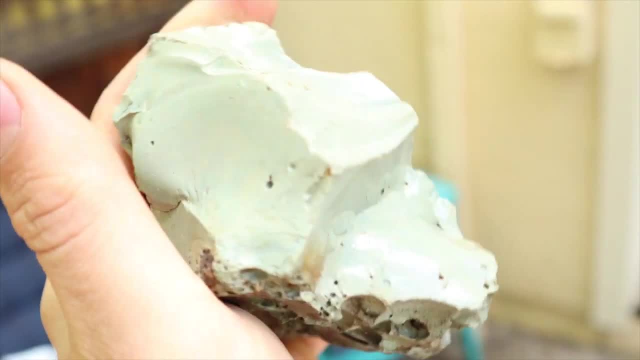 Obsidian, no longer obsidian. so if you see any kind of bubbles which can be very commonly formed in slag glass, You see those. you know right away. It's not going to be obsidian. what you especially want to look for with slag is going to be looking for. 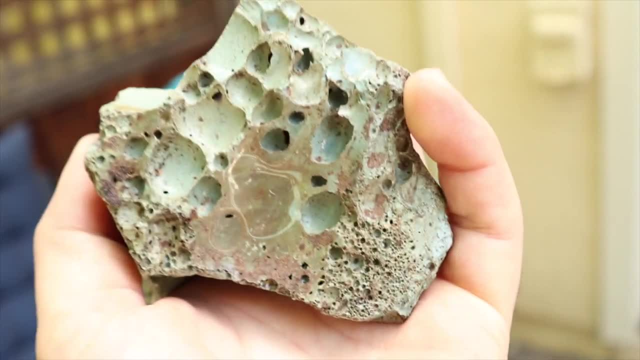 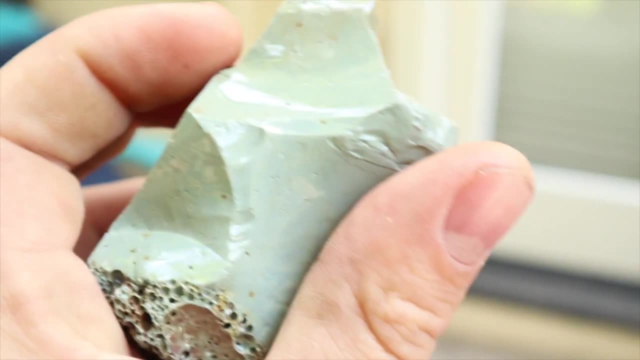 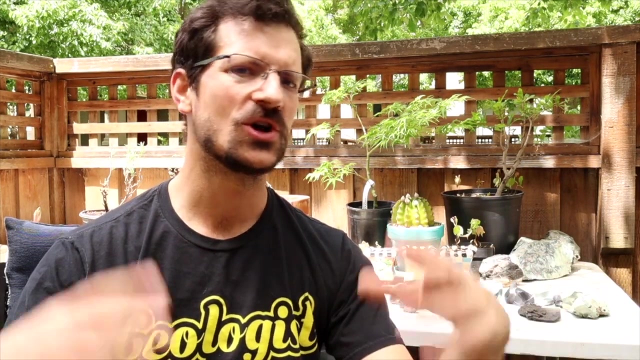 spherical bubbles, perfectly round Bubbles in your in that glass is a dead giveaway, a dead ringer, that it's slag and it is not Obsidian. well, I think that's about it for me here, rock stars, I think I've covered all the important basics that you need to know to go out and tell the difference between slag glass.